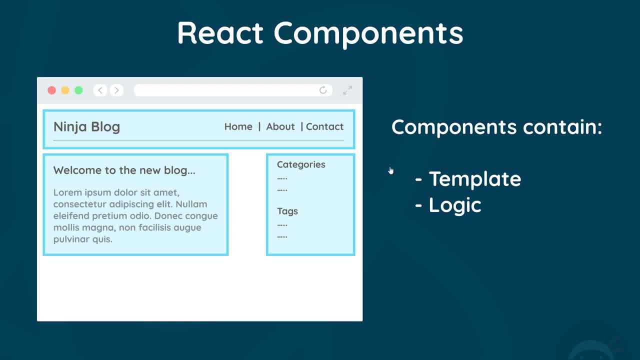 a nav bar component will contain a template which makes up the html for this bit of content, but also any javascript logic, like a function which runs when, maybe, a logout button is clicked. Now, react components allow us to do these things really, really easily. So, to begin with, in our application we only have one single component which is being rendered. 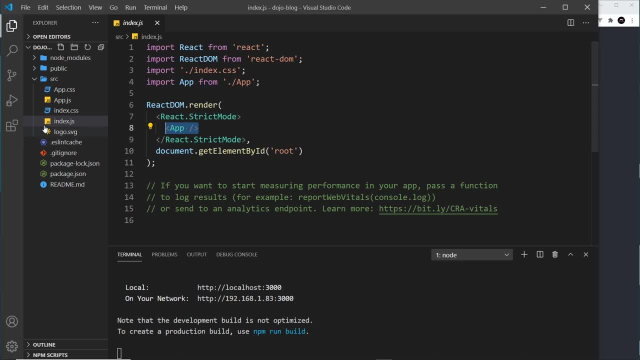 and that is this component right here, app. and, by the way, I'm inside the indexjs file, inside the source folder. This is the file, remember, which kickstarts our application and at the minute, what it's doing is taking this app component right here and it's rendering it to the DOM at this. 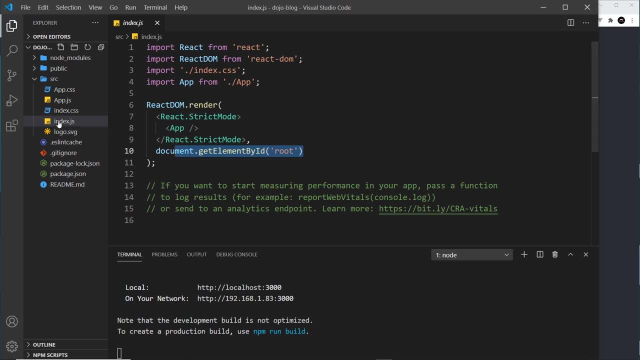 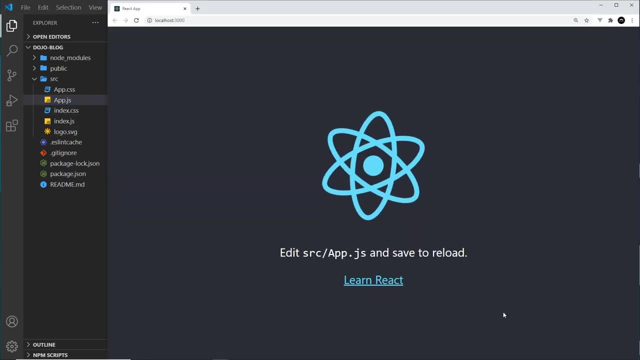 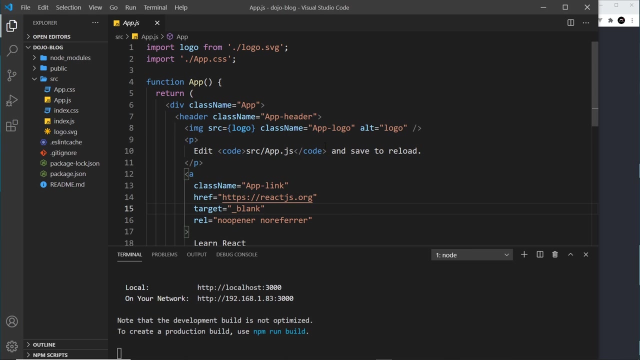 position, So the element with an id of root. So then this component right here, all of the content inside that component is being rendered to the browser and that's what we're seeing right here. All of this content is this content over here. So this component, this is known as the root component. 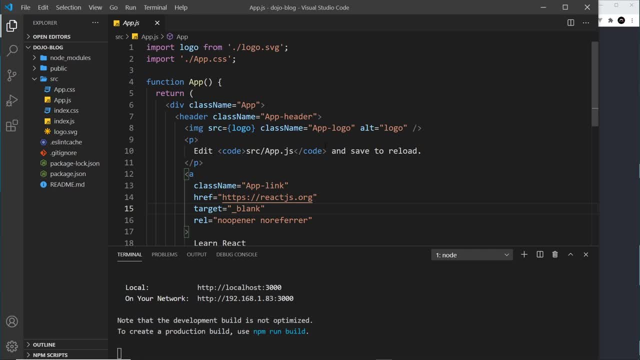 Now. we'll talk more about what a root component means later on, but essentially this is the only component at the minute which is being rendered to the DOM, and inside this component we can see it is being rendered to the DOM. So this is the component which is being rendered to the DOM, and 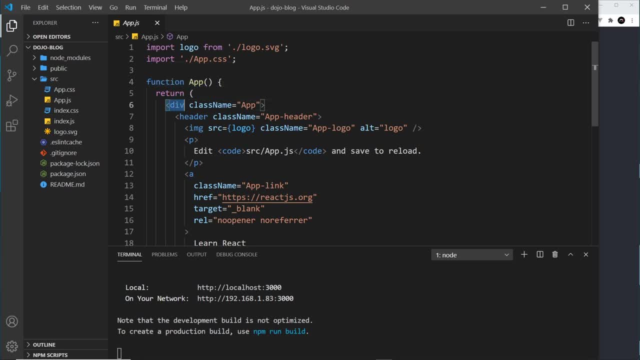 it's basically a function called app and that returns what looks like some HTML code. Now, this function could be an arrow function if you prefer, but it has to start with a capital letter. So this one is called app and it returns this code right here. Like I said, it looks like an HTML template. 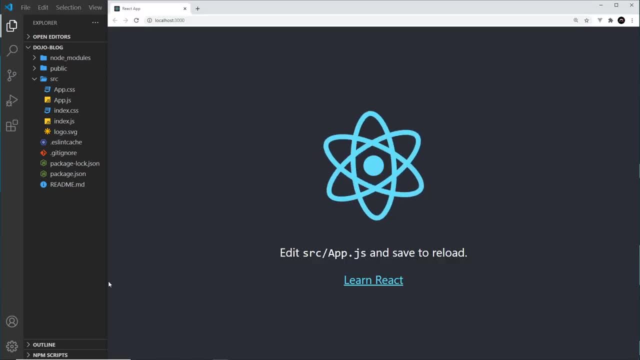 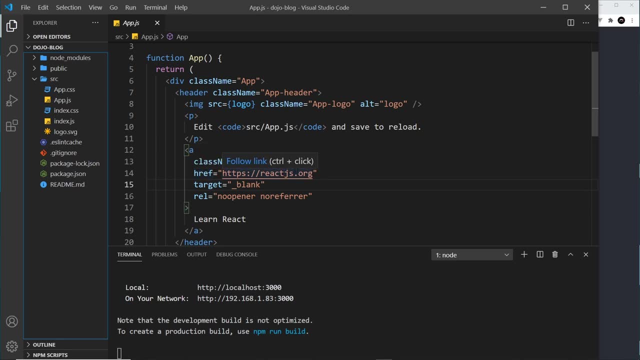 and this is all of the stuff, all of the content we're seeing over here. but this is not actually HTML, It's something called JSX. Now, it has a syntax- all of the content we're seeing over here- almost identical to HTML, but there are some differences which we're going to talk about. 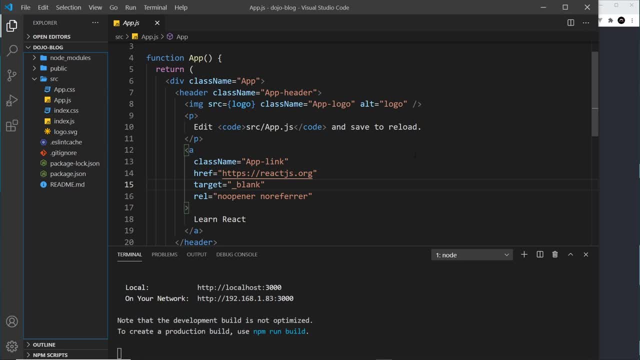 later on. So JSX allows us to easily create these HTML style templates and components, and in the background, a transpiler called Babel converts all of this JSX template into HTML when we save the file and it renders that HTML to the DOM. Okay, so you don't have to worry too. 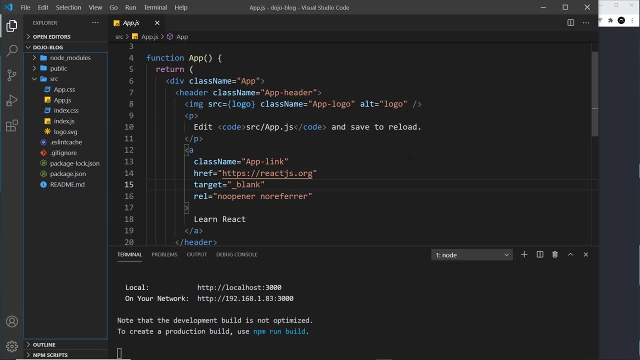 much about how this happens, but just know that this kind of thing is going on in the background, and this template code right here is JSX. Now, one big difference between JSX and HTML is the way we add classes to elements, because in JSX we use this attribute class name and it's also camel case. 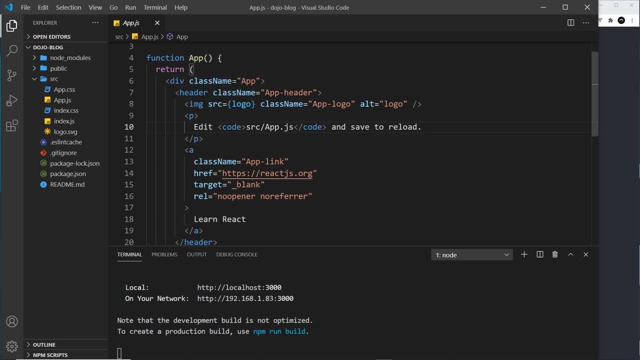 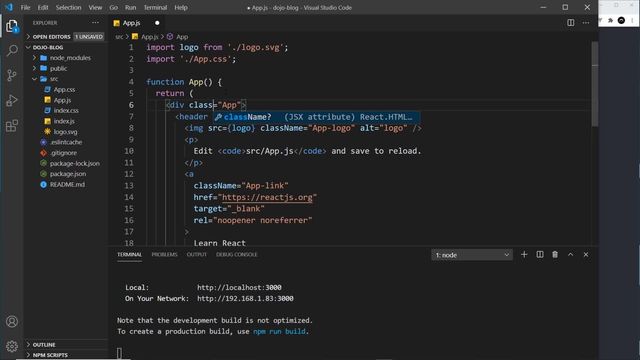 notice: n is a capital. Now, the reason we can't use just class is because class is a reserved keyword in JavaScript and at the end of the day, we're in a JavaScript file right here. so we can't use class name in JSX, and then when this is converted into HTML, it changes this attribute. 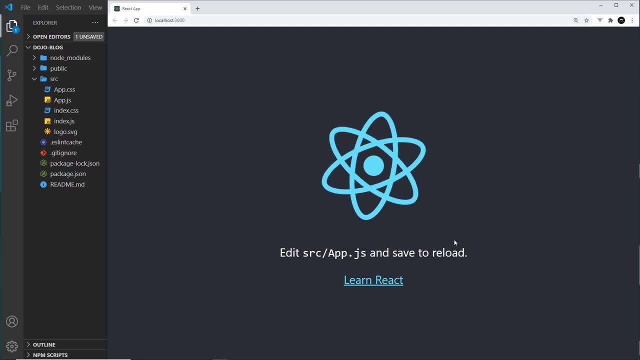 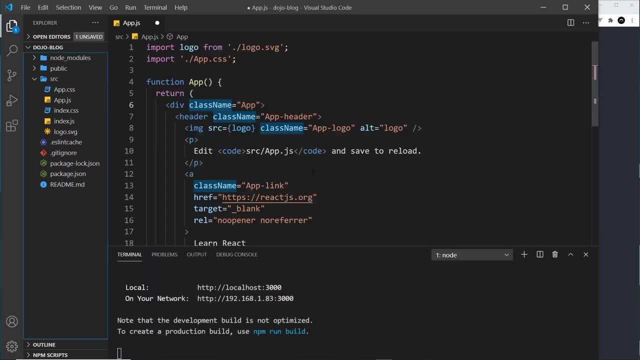 into just class. So if we inspect this over here, we're going to see that it should have a class of app, so it doesn't say class name, just class Okay. so that's one difference, and there are other differences which we'll see later on as well. Now, one thing I want to quickly mention is that in 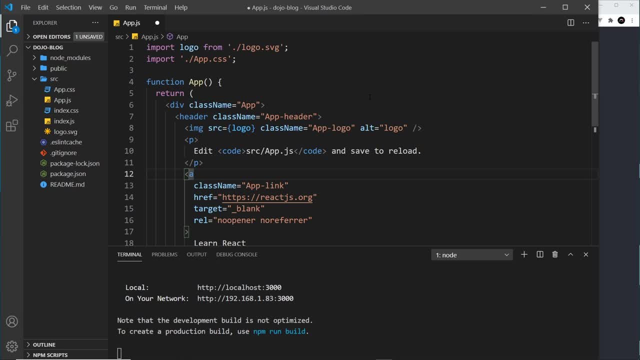 older versions of React, less than version 17.. You need to import React at the top of the file, inside components, for them to work. Notice we don't import React anywhere up here. we input these other things but not React. So if you're using 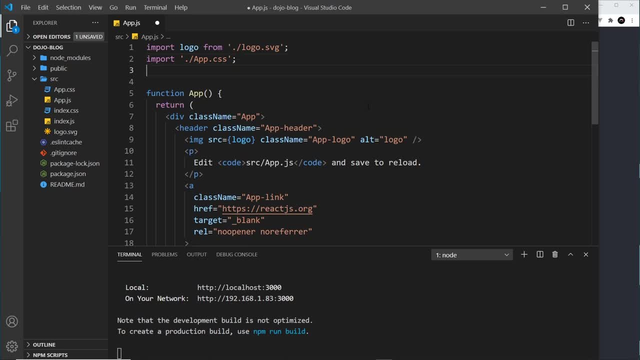 version 16, for example, and not the latest version, for this to work, you might see in your file something like this: import React from React like this, and then this file would work. but in version 17 we don't need to do that, okay, But that's important if you're using an older version. So there's one more thing I want to do in this. 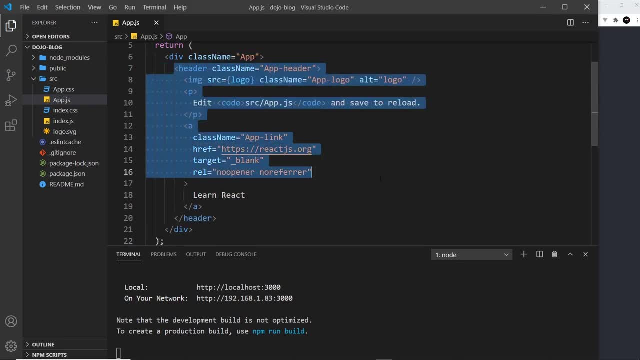 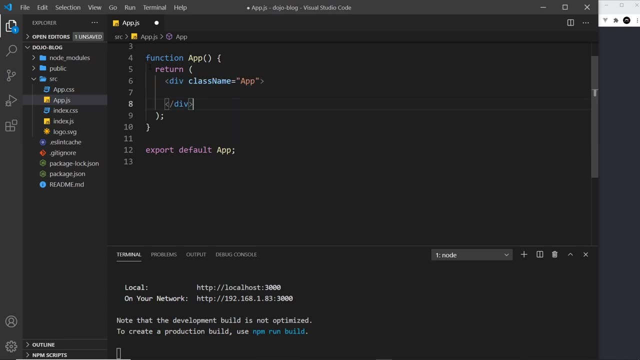 video, and that's to remove most of this template content right here. so everything inside the div with the class name of app will keep this to surround our code. So we have to return this template inside a component right, and now we have this empty div. but I also want inside that a div. 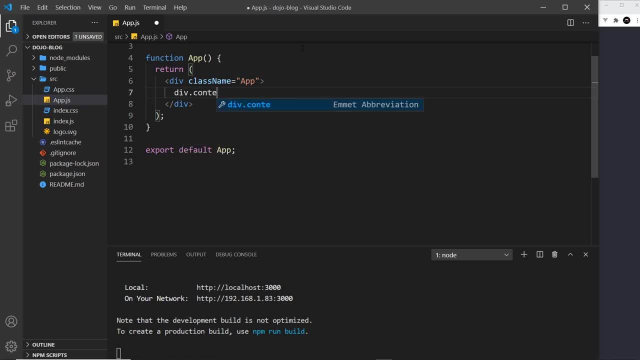 with a class of content. so I'll say divcontent, and this was the MX setup I talked about in the other video in the other class, because now if I press tab it's going to create that div with a class name of content. all right, so inside that I'm going to do an H1 and this is just going to say app.